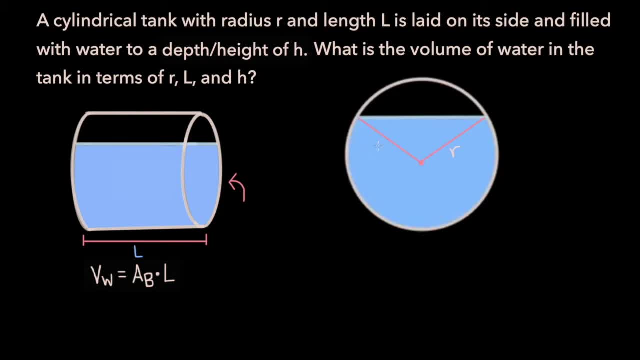 this one. Both of these lines are going to have a length of r, and notice that by drawing these two lines, we split up the shaded region into two different shapes, both of which we can calculate the area of. The first is this triangle and the second is this sector, and so the area of the base. 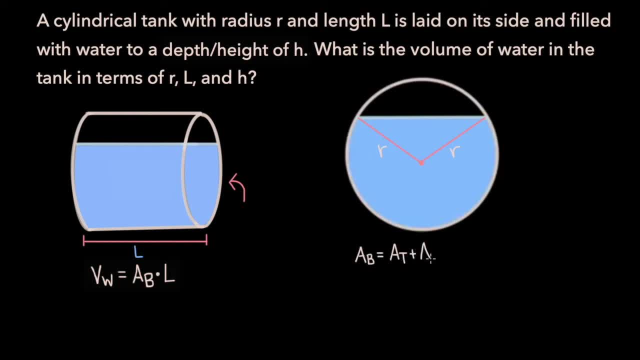 the area of the triangle plus the area of the sector. So let's first work on computing the area of this triangle. To find the area of a triangle, we're going to need to know the length of its base and its height. Let's start by finding its height. We know that the height of the water in our cylinder is. 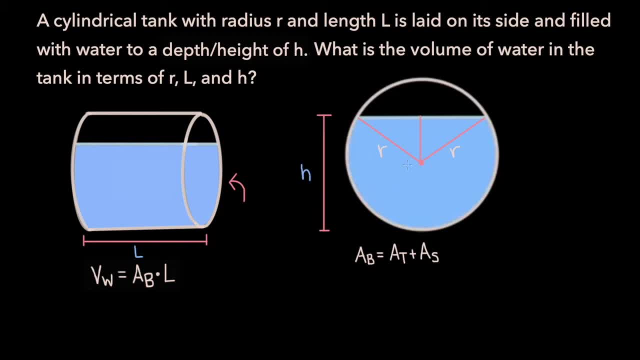 h. The problem tells us that, and we also know the length of this line segment is going to be r, since it's another one of the circle's radii, And so if the height of the water is h and the length of this line is r, 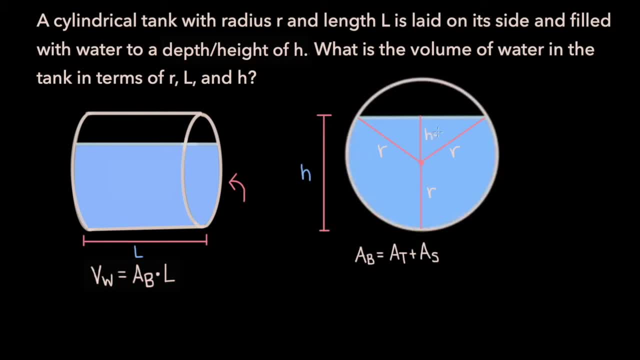 then the height of the triangle must be h minus r. Now imagine for a moment that we split up this larger triangle into two separate right triangles. We can now use the Pythagorean theorem to calculate the length of this leg of the triangle, which we can call a. 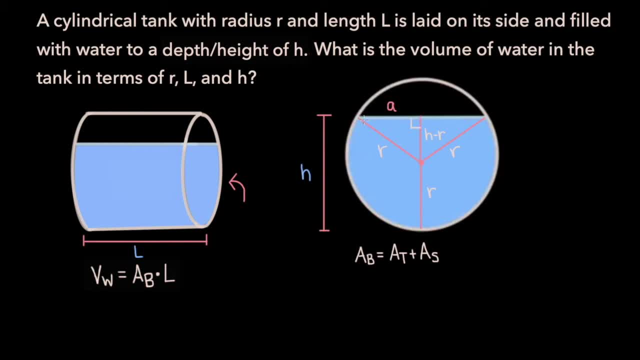 And if we know the length of this leg of the right triangle, then the length of the larger triangle will just be twice that, so 2a. So for the moment let's just use the Pythagorean theorem: on one of these right triangles We get that a squared. 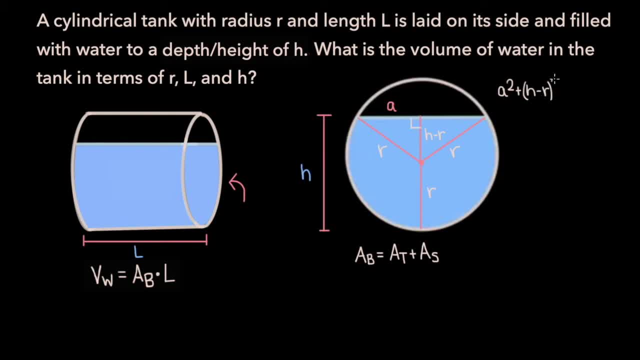 plus h minus r whole squared is equal to r squared. Let's expand the h minus r whole squared term out. We get a squared plus h squared plus r squared minus 2 hr. so this is the h minus r whole squared term expanded out. 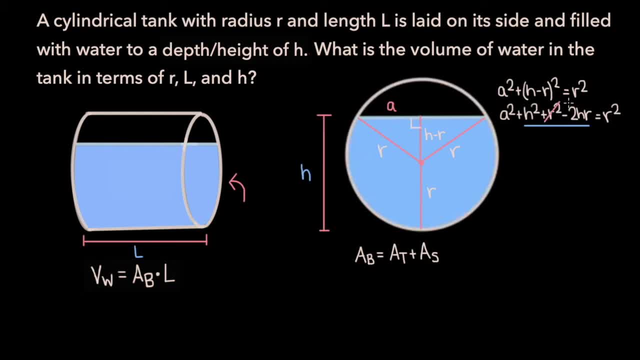 equals r squared. We can cancel out the r squared terms on both sides. and now if we move the h squared and negative 2 hr terms to the right hand side, we get a squared is equal to 2 hr minus h squared. Now let's take the square root of both sides. we get a on the left hand side. 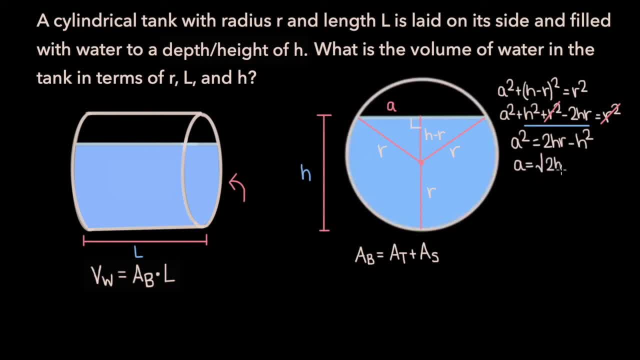 and on the right hand side we have the square root of 2 hr minus h squared, and if that's the length of a, which is the leg of one of these right triangles, then the length of the base of the larger triangle will be two times that, so two times the square root of 2 hr. 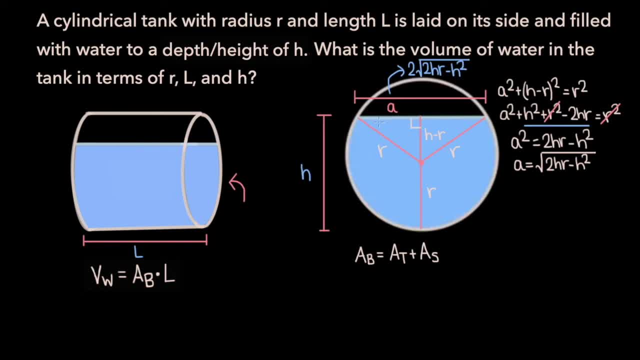 minus h squared. Now that we know the lengths of the base and height of this larger triangle, we can find its area. So the area of the triangle is going to be equal to one half base times height, so one half times the base, which is two times the square root of 2 hr minus h squared. 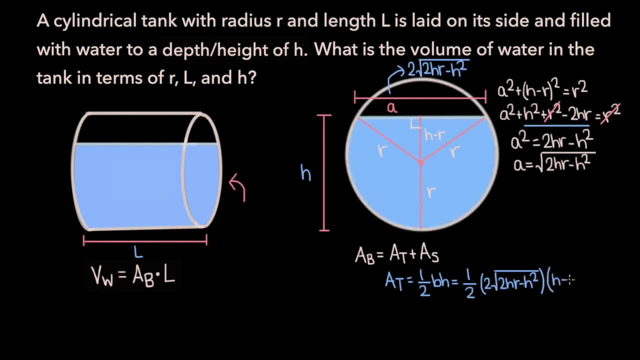 times the height, which is h minus r. The two in the numerator and the two in the denominator will cancel, and so we get that the area of the triangle is equal to the square root of 2 hr minus h, squared times h minus r. Now let's work on finding the area of this sector. Now, this sector is just a. 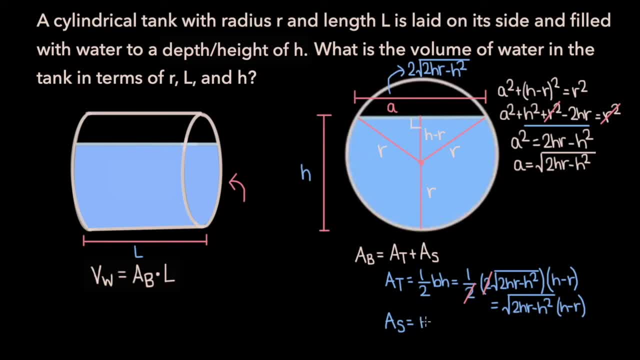 portion of the circle. so to find its area, we're going to take the area of the circle which is pi r squared and multiply that by whatever fraction. this angle is out of 2 pi radians. So if we call this angle alpha, 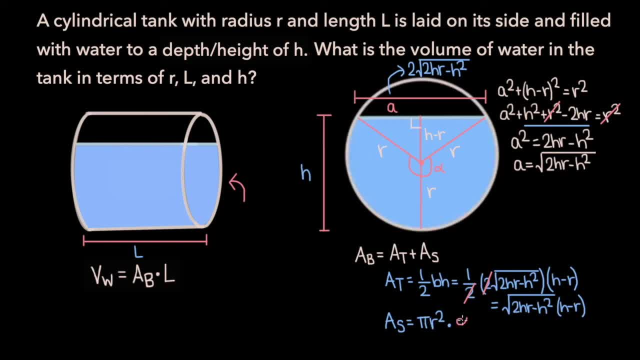 then the area of the sector is going to be pi r squared times alpha over 2 pi, assuming that we're working in radians. Well, to find out what alpha is, we're going to need to know what this angle is. Let's call that theta. What do we know about theta? Well, we know that. 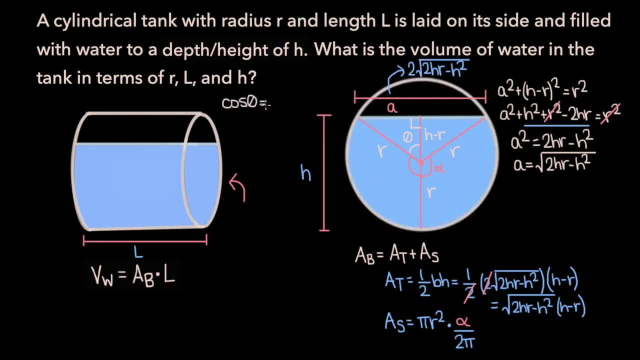 cosine, theta is going to be adjacent over hypotenuse, so h minus r over r, and so theta is going to be equal to the arc cosine of h minus r over r. If this angle is theta, then we know that this angle must be theta as well. 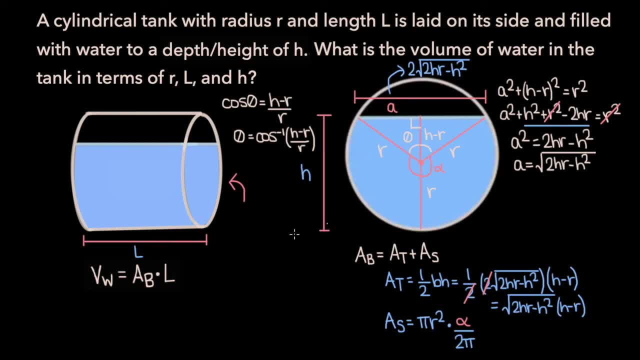 since the two right triangles are identical and so alpha- if we just bring this down here for the sake of space, alpha will be equal to the angle measure of the entire circle, which is 2 pi, if we're thinking in terms of radians minus 2 times theta, so 2 times the arc cosine of h minus r over r. 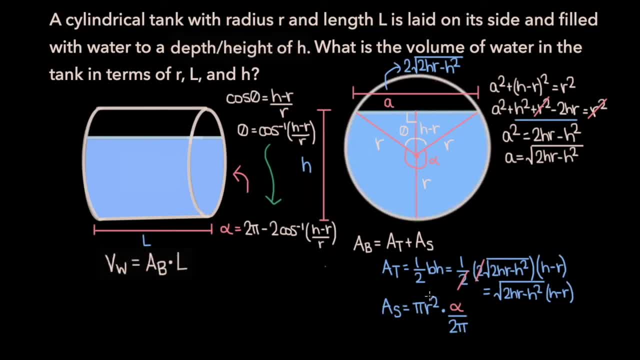 And so now, if we return to the formula for the area of a sector, let's do some simplification. We can cancel out the pi in the numerator with the pi in the denominator, and then we're going to have r squared times alpha over 2.. Now we can factor out a 2 in our formula for alpha. 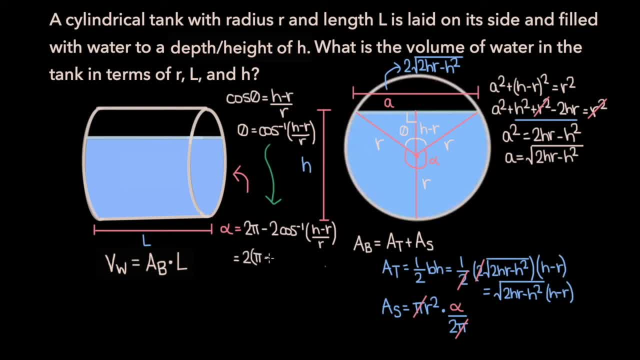 and we would get 2 times pi minus the arc cosine of h minus r over r, And so the area of the sector will be r squared times alpha, which is 2 times pi minus the arc cosine of r2.. of h minus r over r, all over two, We can cancel out a two in the numerator with the two in the. 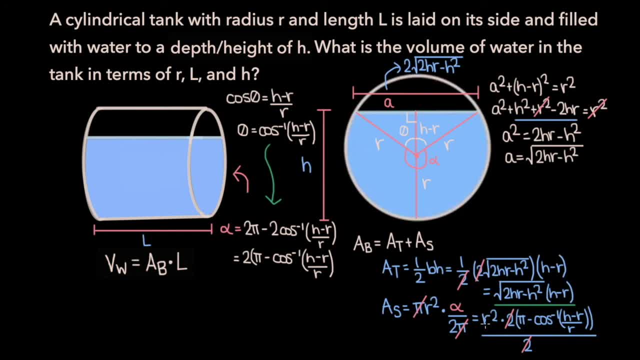 denominator and we're left with the area of the sector as r squared times pi minus the arc cosine of h minus r over r. Now we know the area of the triangle and the area of the sector. so we know what the area of the base is. So now we just have to put everything together to get a formula for. 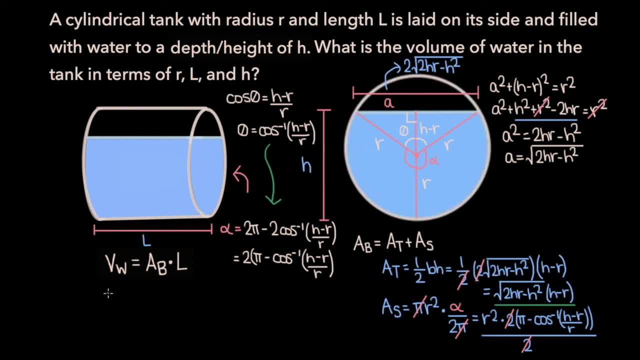 the volume of water in a horizontal cylindrical tank. So the volume of the water is going to be equal to the area of the base, which is the area of the triangle, plus the area of the sector. The area of the triangle is the square root of two h r minus h squared times h minus r plus the area. 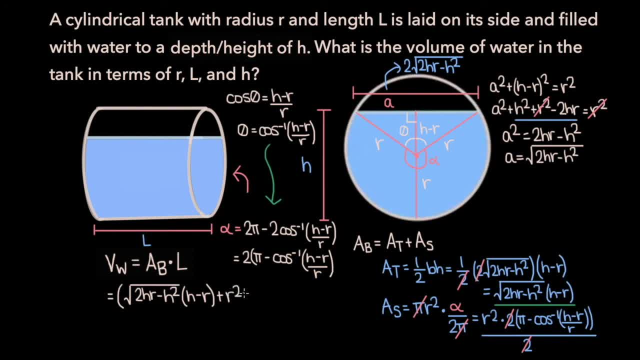 of the sector, which is r squared times pi minus the arc cosine of h minus r over r. and if we close our parentheses, and so this is the area of the base, Then to get the volume of the water we're going to need to multiply that quantity by the length. 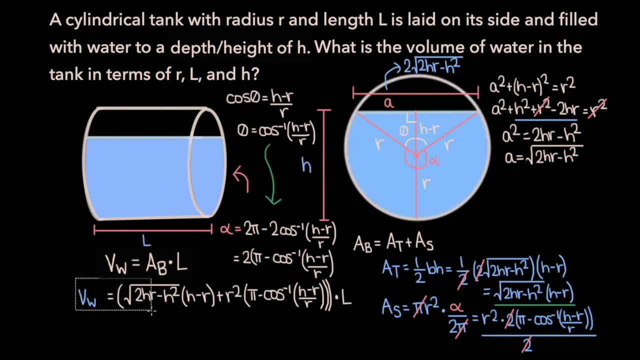 of the cylinder, which is l. So here's the formula you can use to determine the volume of water in a horizontal cylindrical tank, where r is the radius of the tank, l is the length of the tank and h is the depth to which water is filled. 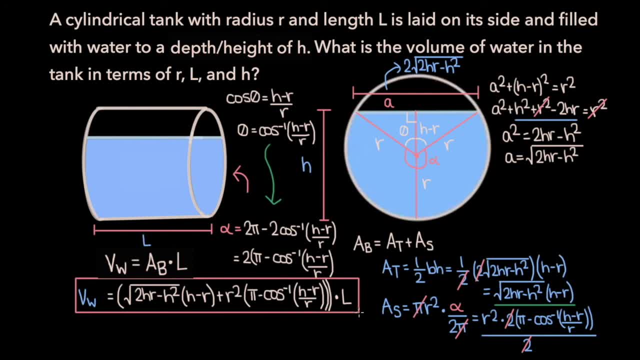 All right, that wraps it up for this video. If this video did help you out, please do consider leaving a like and subscribe if you want to be notified when I post more content like this. Thanks for watching.